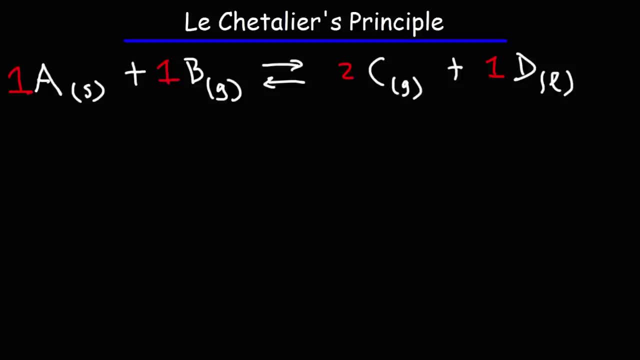 when a chemical reaction is in equilibrium- it's not static equilibrium where everything is stationary- We have a case of dynamic equilibrium. That means things are moving. When we have dynamic equilibrium, the rate of the forward reaction is going to be equal to the rate of the reverse reaction, Because these two reactions are 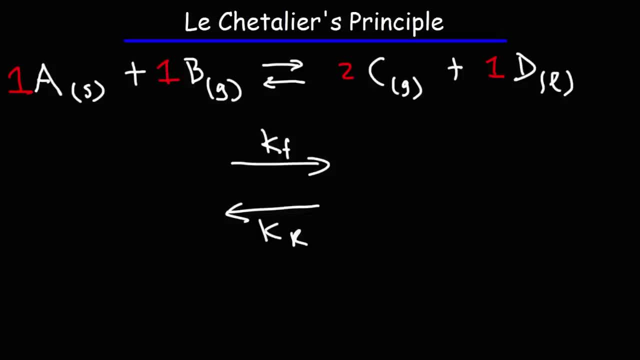 occurring at the same rate, there's not going to be any net change in the amount of product and reactants. So the concentration of the products and reactants: they remain constant at equilibrium because the rate of the forward reaction equals the rate of the reverse reaction. 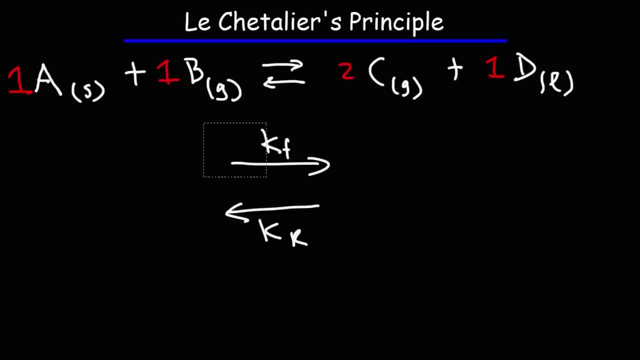 So that's the situation that we have at equilibrium. Now let's consider what's going to happen if we add stress to the system. So let's increase the concentration of reactant B If we introduce more of substance B to the vessel, if we increase its concentration. 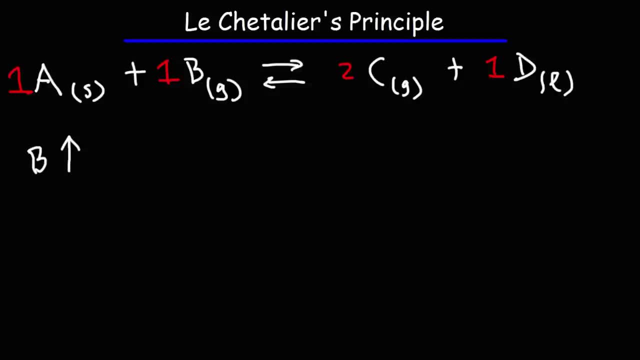 what's going to happen to this reaction? Will the reaction shift towards the right, that is, towards the products, or will it shift towards the products? It's going to shift towards the left, towards the reactants. So think of the concept of equilibrium. 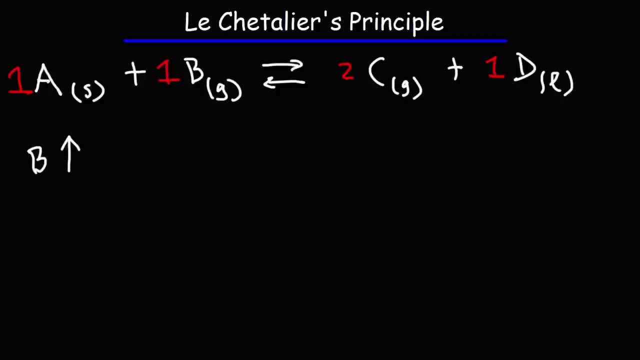 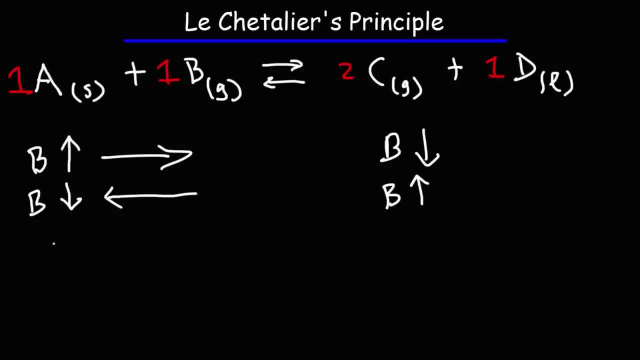 If the reaction shifts to the left, the products will increase. If it shifts to the left, the products will increase. If the reaction shifts to the left, the products will increase. If it shifts to the left, the products will increase. Let's focus on the products. Let's say that if we increase the concentration of C, 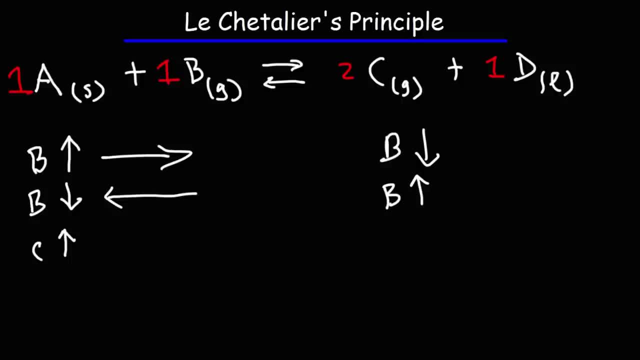 What's going to happen? Will it shift to the right or to the left? Now, C is the product. If we increase it, the system is going to try and decrease it. In which direction should the reaction shift in order to decrease the concentration of? 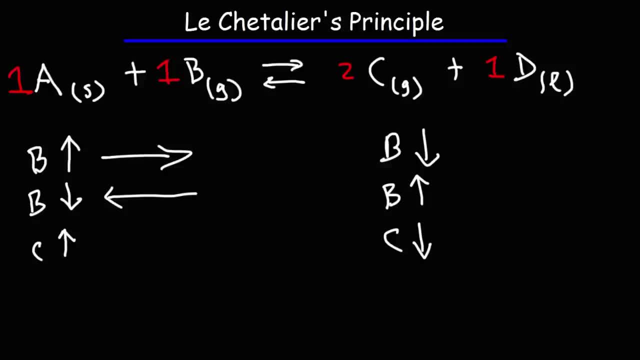 C, Or you could say the partial pressure of C, since it's a gas. If the system were to shift to the right, we know, the reactants would go down, the products would go up. C is a product. The system is not trying to increase the product. 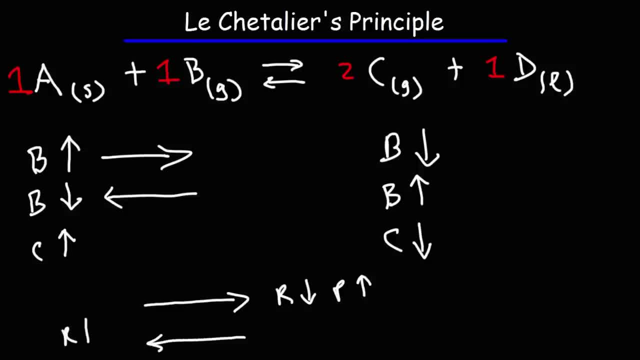 It wants to decrease it. so it has to shift to the left, Where the reactants would go up, the products would go down. So if you increase C, the system is going to move away from C to decrease it. Whenever the system moves away from a reactant or a product, that product or reactant is going to go down. 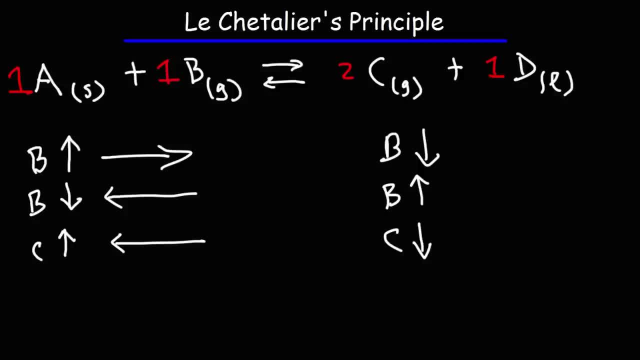 When the system moves towards it, it's going to go up. So let's say, if we were to decrease C, the system is going to try to increase C. In order for the system to increase the concentration of C, it has to shift towards the products, so it's going to shift towards the right. 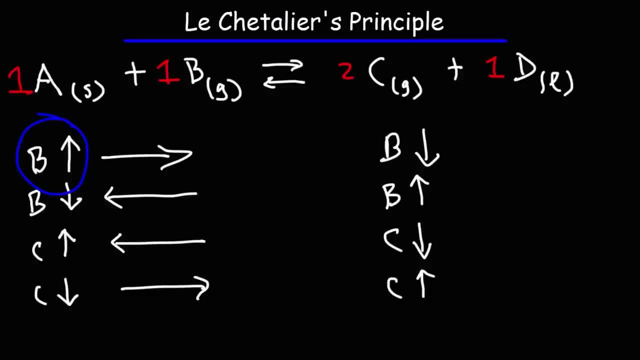 So to review: if you were to increase the reactants, the reaction is going to shift to the right. If you were to increase the products, the reaction is going to shift to the left. Now, what's going to happen if we increase reactants? 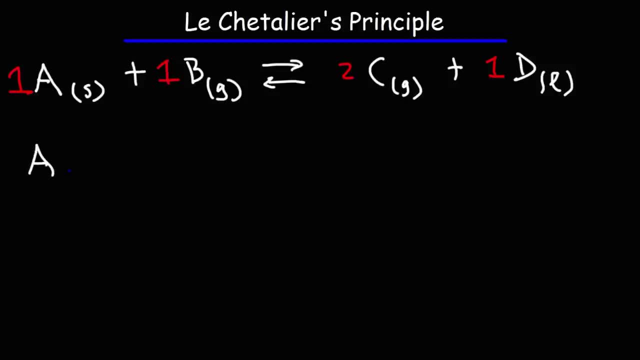 Let's say, if we introduce substance A or more of substance A into the reaction vessel, What's going to happen to the reaction? Will it shift to the right or to the left? A is in the solid state. As a result, increasing A will have no effect on the position of equilibrium. 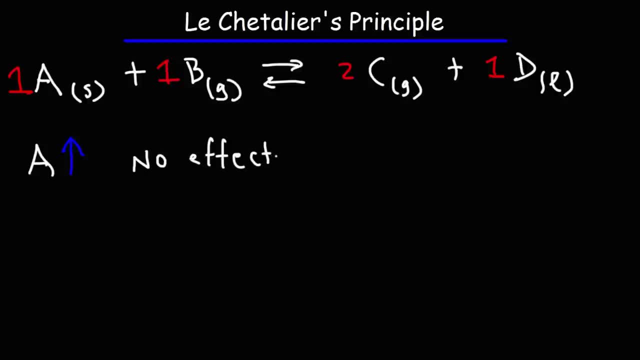 The reaction will not shift to the right, nor will it shift to the left. Now, if you recall, the equilibrium constant K is equal to the concentration of the products divided by the concentration of the reactants. Notice that A and D are not included in the equilibrium expression. 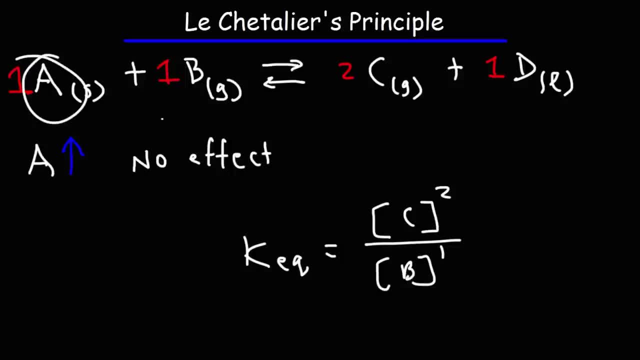 The equilibrium constant does not depend on the value of A or D, because they're in the solid and liquid phase. The only thing that will affect K is gases or substances in the gas phase or substances dissolving in the aqueous phase. 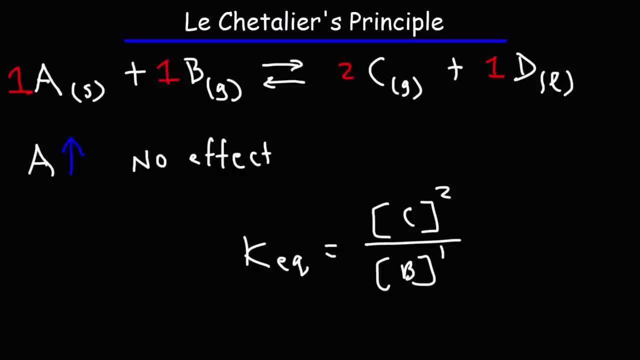 So if it's not dissolved in an aqueous solution or if it's not a gas, it's not going to be included in the equilibrium expression. So changing the value of a solid or a liquid, it's not going to have any effect on the position of equilibrium. 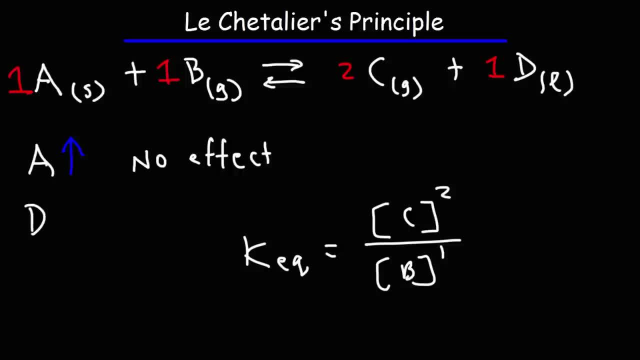 So if we were to increase D, let's say if we were to add more of substance D, this will have no effect on the position of equilibrium. Adding more liquid to the reaction vessel, it's not going to affect these two reactants. 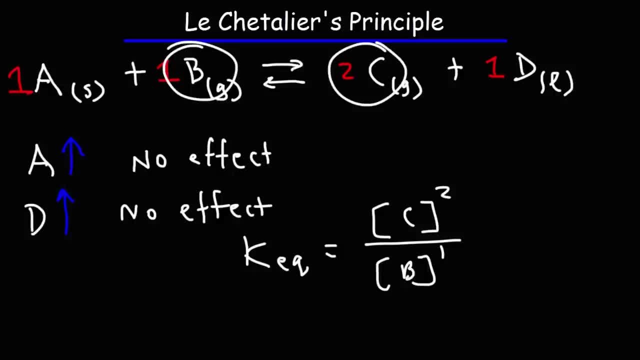 I mean it's not going to affect B or C because they're in the gas phase, So they're outside of the liquid. Therefore, to summarize, increasing or decreasing any reactant or product in the solid or liquid phase will have no effect on the position of equilibrium. 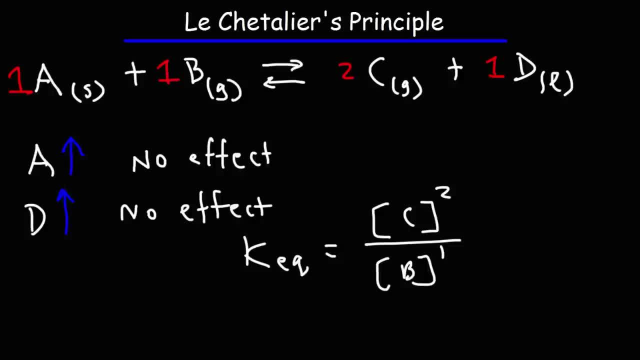 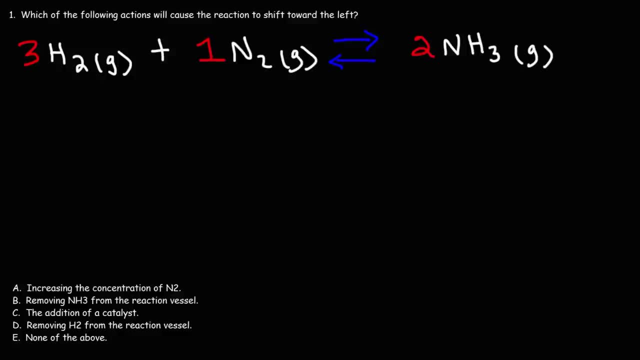 So just keep that in mind. But now let's go ahead and work on some practice problems. Number one: which of the following actions will cause the reaction to shift toward the left? So let's analyze each answer choice. So what's going to happen if we increase the concentration of nitrogen gas? 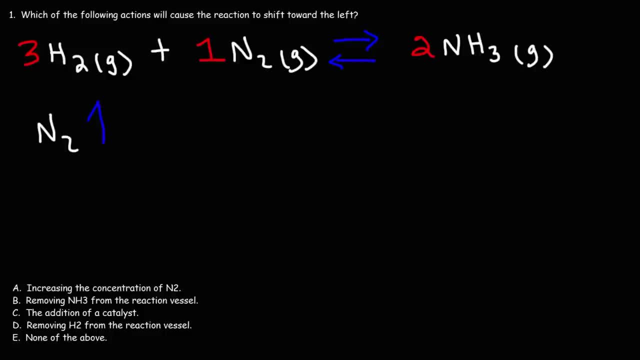 Nitrogen gas is a reactant. If we increase the concentration of the reactant, the system is going to try to undo that change. It's going to try to bring the concentration of N2 back down. And remember, any time the reaction shifts towards the right, the reactants will go down. 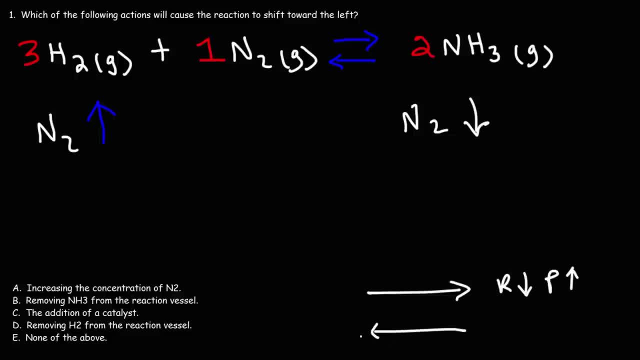 The products will go up. If the reaction shifts to the left. the reactants go up but the products go down. N2 is a reactant, So it's going to go in a direction to decrease that reactant, So it's going to shift towards the right. 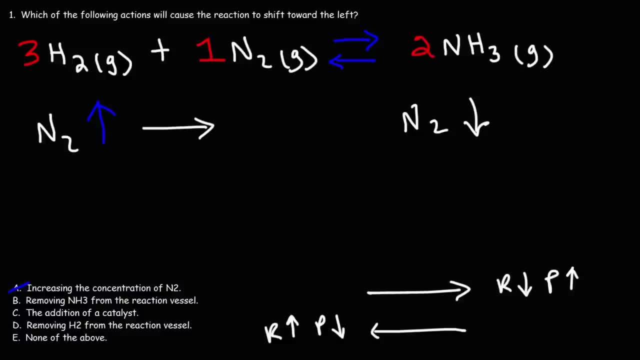 So thus we can eliminate answer choice A because it's going towards the right. Now, what about B? Let's say if we were to remove NH3 from the mixture. So if we're decreasing the concentration of NH3, in what direction will the reaction shift? 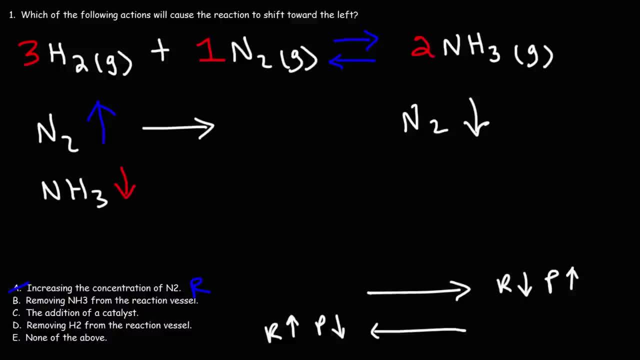 Well, according to Le Chatelier's principle, we're decreasing the product, The reaction is going to try to increase that product. So in order to increase the product, it has to shift to the right. So we can also eliminate answer choice B. 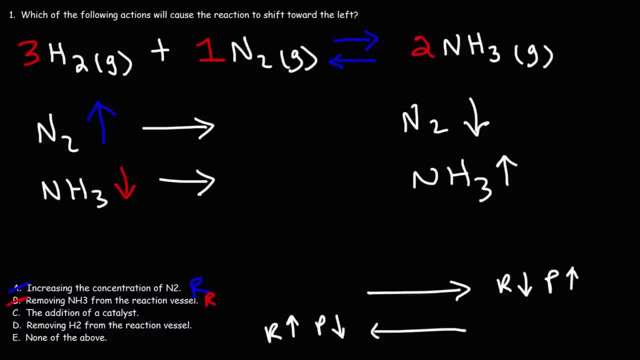 So we can also eliminate answer choice B, since it's going to the right. Now, what about C, The addition of a catalyst? If we were to add a catalyst, what's going to happen? Will the reaction shift to the right or to the left? 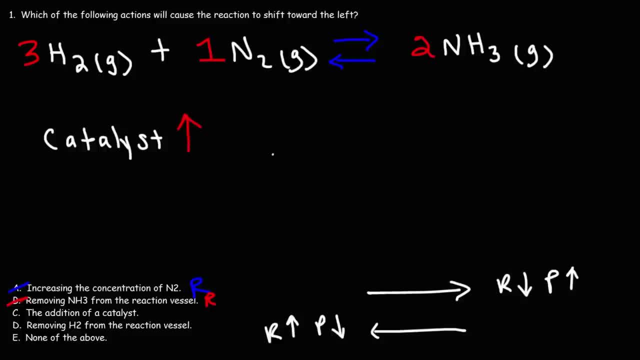 The addition of a catalyst will cause the reaction to speed up, So the reaction is going to go towards equilibrium at a faster rate. A catalyst works by speeding up the rate of the forward reaction, So it's going to increase Kf, but it also increases the rate of the reverse reaction. 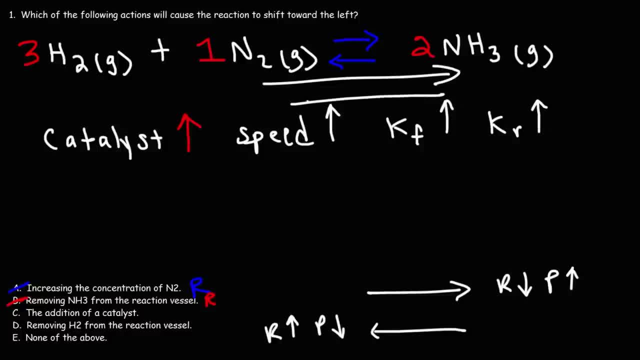 So the reaction is going to go to the right at a faster rate, but it's also going to go to the left at a faster rate. Thus it's not going to change the concentration of the products in the reactants, Because the relative concentration of the products in the reactants 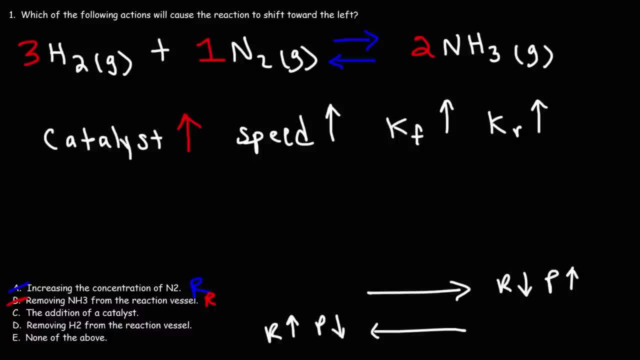 won't change because there's no net change by introducing the catalyst. the catalyst has no effect on the position of equilibrium. Even though it speeds up the reaction in both ways, it doesn't shift it to the right, nor does it shift it to the left. 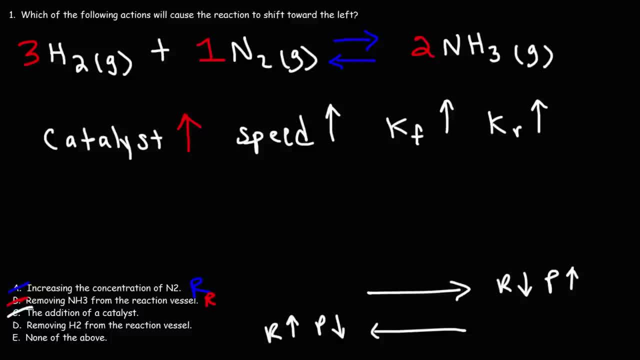 So it has no effect. So C is out. So remember: a catalyst simply speeds up a chemical reaction. It has no effect on the position of equilibrium. Now, what about removing hydrogen gas from the reaction vessel? What's going to happen if we decrease the amount of hydrogen gas by taking it out of the reaction? 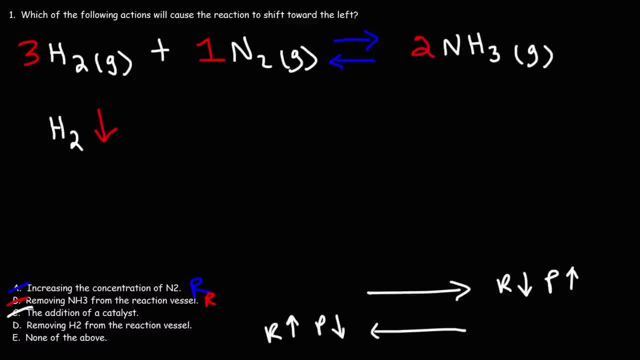 So hydrogen gas is a reactant. If we decrease the amount of hydrogen gas, the system is going to try to do the opposite. It's going to try to increase. So it's increasing a reactant. Now, what must the system do in order to increase the reactant? 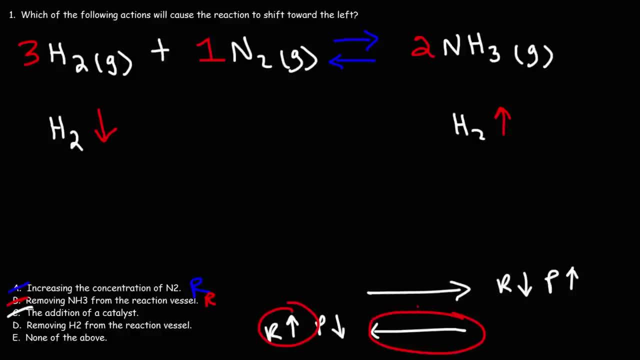 The only way it can increase the reactant is by shifting to the left, And that's what's going to happen. So if we remove H2, the system is going to try to produce more of H2.. Therefore, D is the answer that we're looking for. 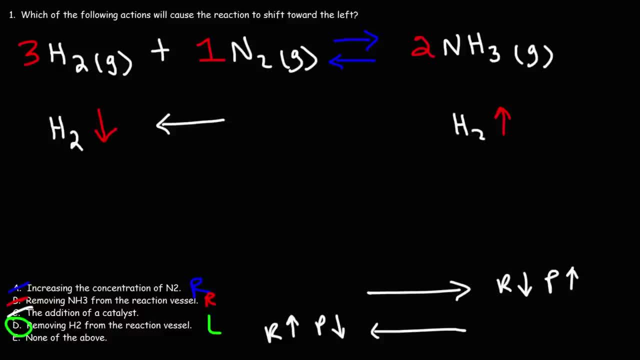 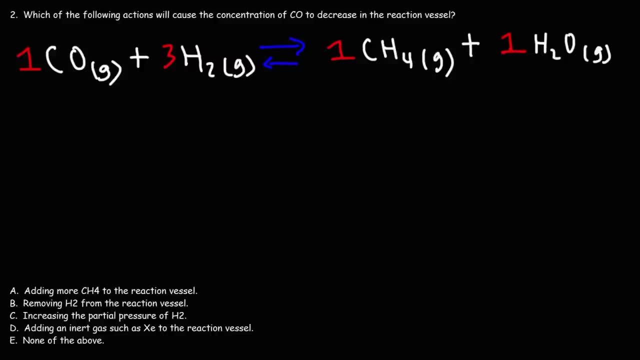 So that's the action that will cause the reaction to shift towards the left. It's by decreasing one of the reactants, Number two. Which of the following actions will cause the concentration of CO to decrease in the reaction vessel? So let's look at each answer choice. 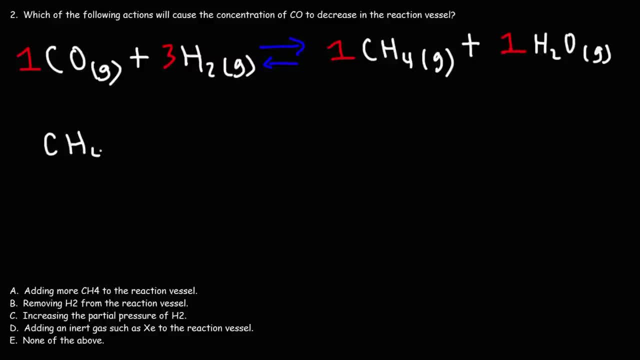 If we were to add more CH4 or more methane to the reaction vessel, what's going to happen? As we increase the concentration of the product, the reaction is going to shift to the left. It's going to move away from the product side. So as to decrease methane. Remember, if it shifts to the left, that is, towards the reactants, the reactants will go up. It's moving away from the products, So the products will go down As it shifts to the left. 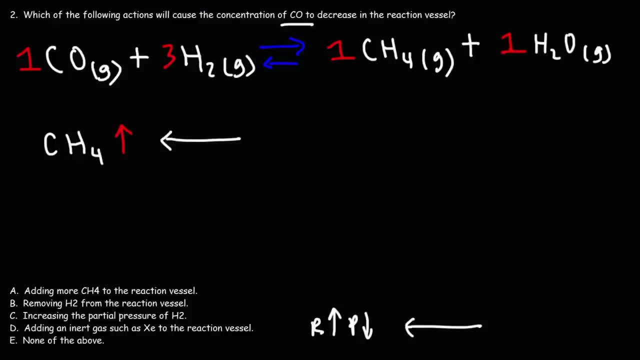 what's going to happen to CO? What will be the effect of CO? Now, CO is a reactant, So when a reaction shifts to the left, CO is going to increase. Methane being a product is going to decrease. So, since you increase methane, 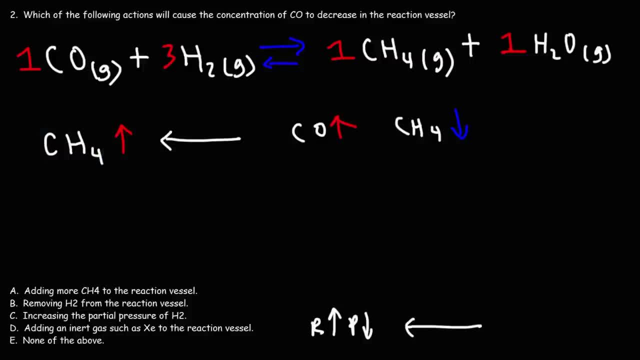 the system is going to try to decrease it And as it shifts to the left, the effect on CO is that it's going to increase. So, since CO is not decreasing, A is not the answer we're looking for Now. what about B? 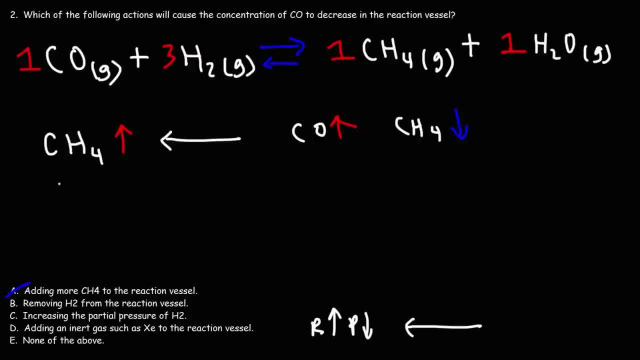 Removing H2 from the reaction vessel. So if we were to decrease the concentration of hydrogen gas, what's going to happen? Hydrogen gas is a reactant And as you decrease hydrogen, the reaction is going to shift towards it. Remember: 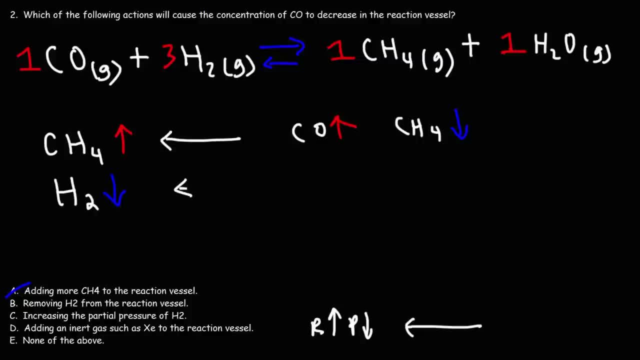 the system is going to try to do the opposite of what you did to it. So because you added hydrogen, the system wants to. I mean, because you removed hydrogen, the system wants to increase it back to its original level, Or at least somewhere closer to its original level. 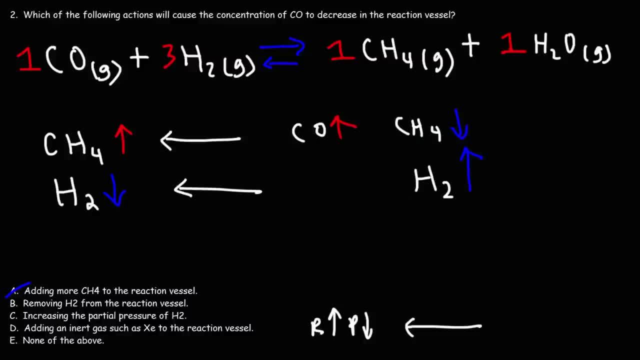 So the reaction is going to shift towards it. Remember, the system wants to increase the reactant closer to its original level. The only way it's going to increase the reactant is by shifting to the left, which is what's going to happen. 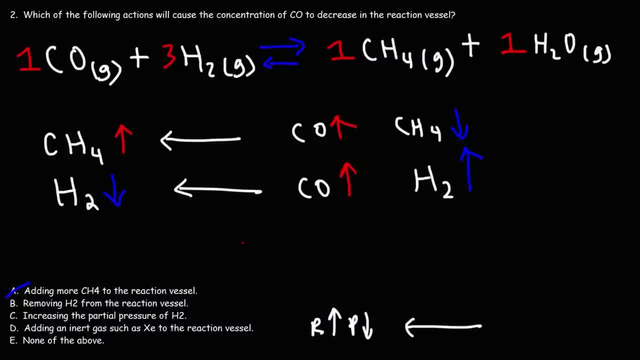 And as it shifts to the left, the concentration of CO is going to go up again. So B is not the answer we're looking for. It's not going to decrease the concentration of carbon monoxide. Now what about answer choice C? 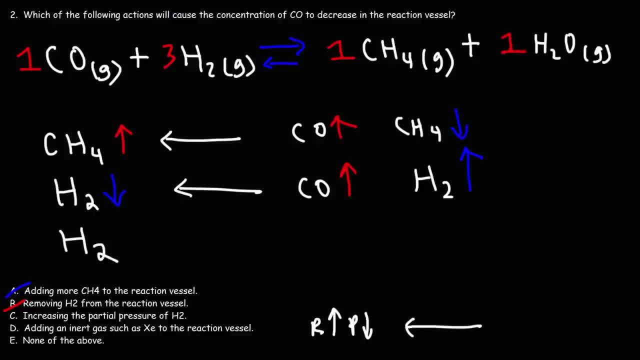 What's going to happen if we increase the partial pressure of hydrogen gas? Now, before we answer that question, I want to mention a few things. When speaking in terms of a reactant or a product that's dissolved in the aqueous solution, the term partial pressure doesn't apply. 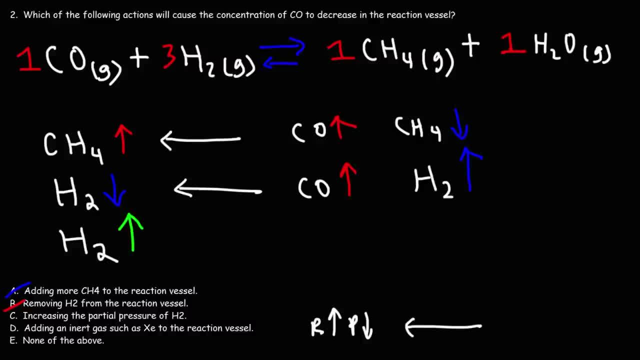 because it's not a gas. However, we can describe it in terms of its concentration, But when dealing with gases, you can talk about it with reference to partial pressure, since all gases exert some level of pressure, But you can also talk about it in terms of concentration. 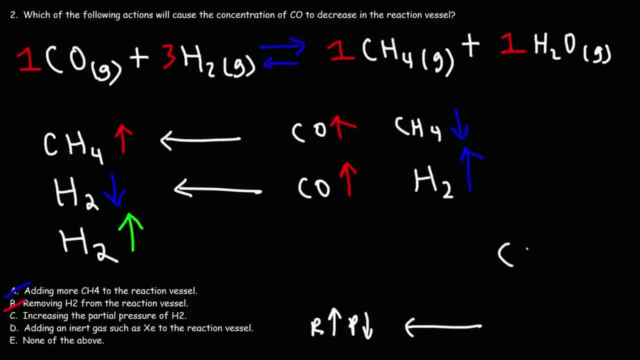 Because in a reaction vessel there's going to be some number of moles of a particular gas in a certain volume. The reaction vessel will have some amount of volume to it, Either a 2 liter vessel or a 3 liter vessel, So you can describe a gas in terms of. 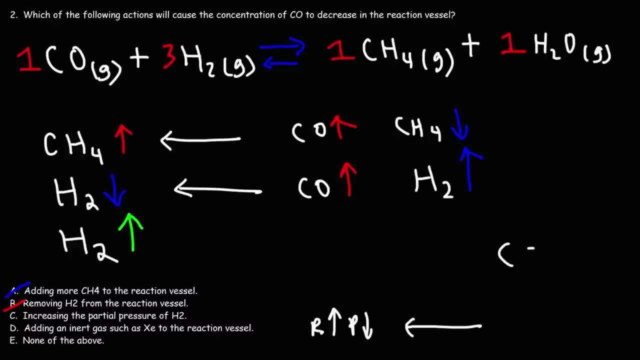 concentration and in terms of partial pressure. Now, as we introduce more hydrogen gas to the reaction vessel, the concentration of hydrogen goes up, and the same is true for the partial pressure of hydrogen. Both goes up, So the effect of increasing H2 will have. 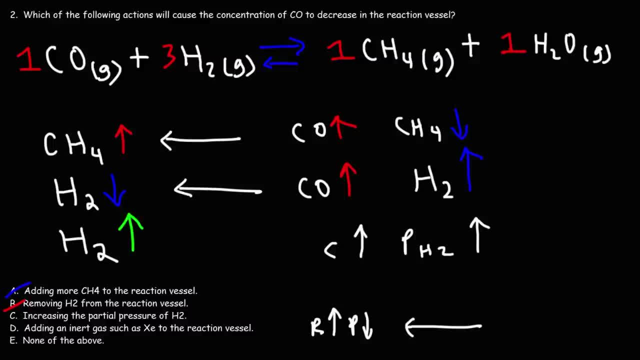 the same effect as increasing the partial pressure of H2.. They will cause the reaction to shift in the same direction. So, whether we're increasing the concentration of H2 or increasing its partial pressure, the only way we can achieve that is by adding more H2.. 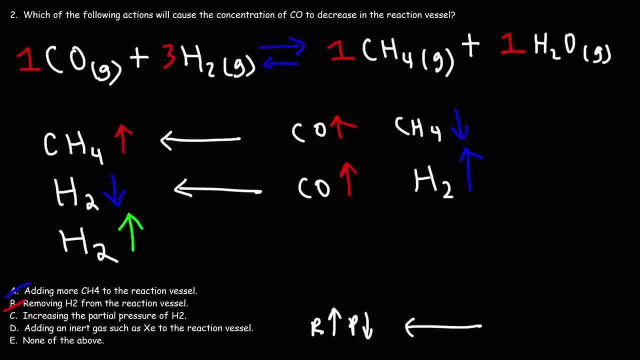 to the reaction vessel. So what's going to happen as we add H2? As we increase the reactant, the system is going to try to decrease the reactant. It can only do that by shifting toward the products, Where the products will go up and the reactants 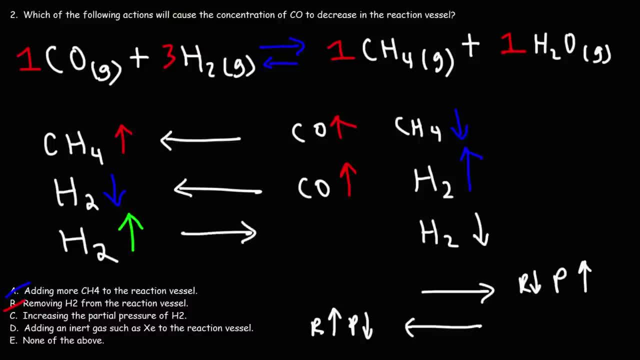 will go down. So it's going to shift to the right. And as it shifts to the right it's moving away from CO, CO being a reactant. So this time CO is going to decrease in value. So that's how we can cause the concentration of CO. 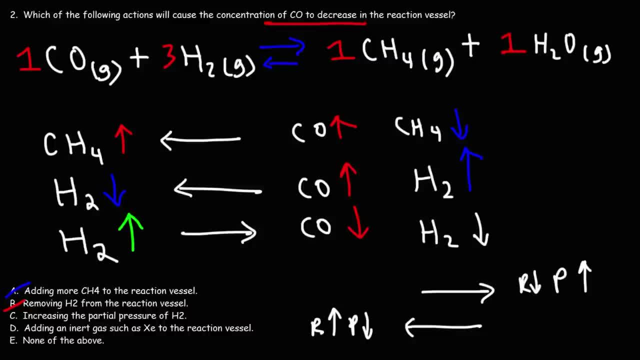 to decrease, We need the reaction to shift to the right, away from the reactants, causing this to decrease while the products go up. So answer choice C is the correct answer. So here's a good way to remember this. In a reaction, we have the 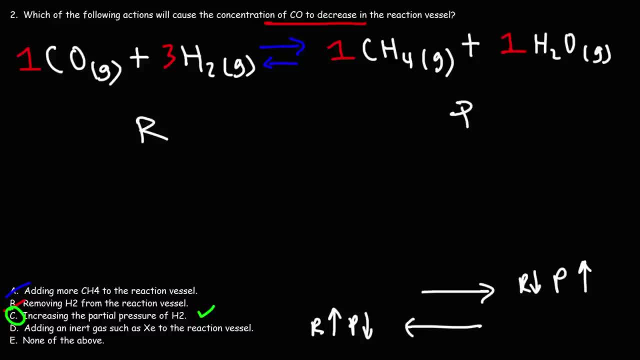 reactants on the left, the products on the right. Now let's say the reaction is shifting towards the right. Notice that it's shifting towards the product side. Therefore, the products should increase in value, And it's shifting away from the reactant side. Therefore, the 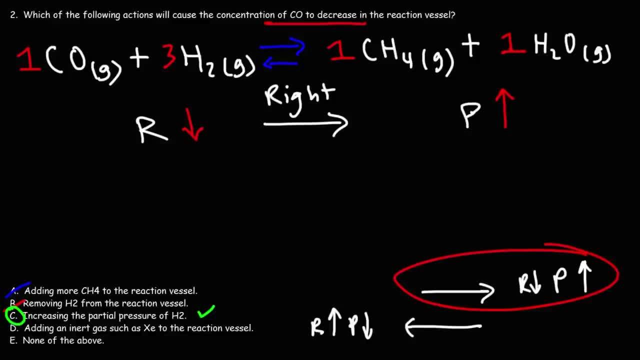 reactants will decrease. So that's a good way to remember what happens there. when it shifts to the right, When it shifts to the left, notice that it's shifting toward the reactants. So, in whatever direction, equilibrium shifts towards where the arrow points. 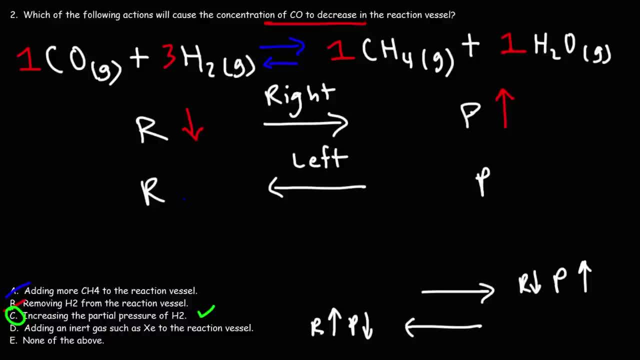 that's what's going to go up. So as it shifts to the left toward the reactants, the reactants is going to go up in value And it's shifting away from the products, so the products will go down in value. So that's a good way to remember. 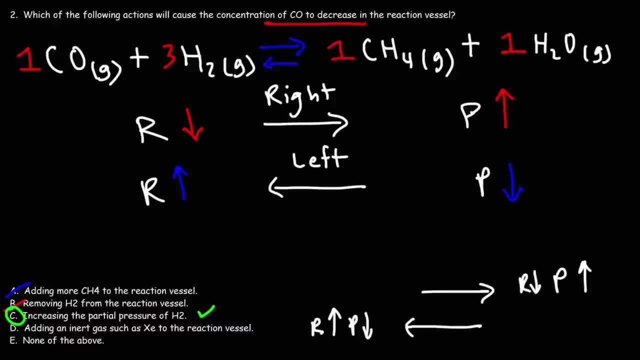 what happens to the reactants in the products when the system either shifts to the right or to the left. Now let's look at answer choice D for the sake of understanding What happens if we were to add an inert gas such as neon. I mean xenon. 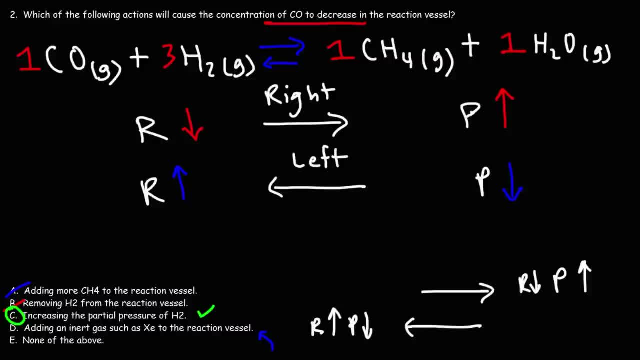 rather to the reaction vessel. Neon is also an inert gas, So this can be true of any one of the noble gases: Helium, neon, argon, xenon, krypton. They're all inert gases. What's going to? 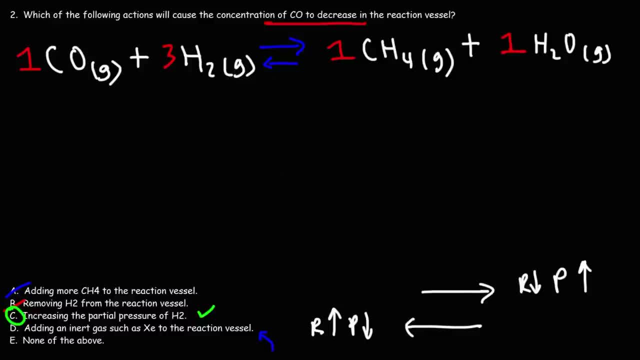 happen if we add an inert gas to this reaction. So if we were to introduce xenon, xenon doesn't react with any of the reactants, nor does it react with any of the products, And it's not in this reaction. It's not included in the equilibrium expression. 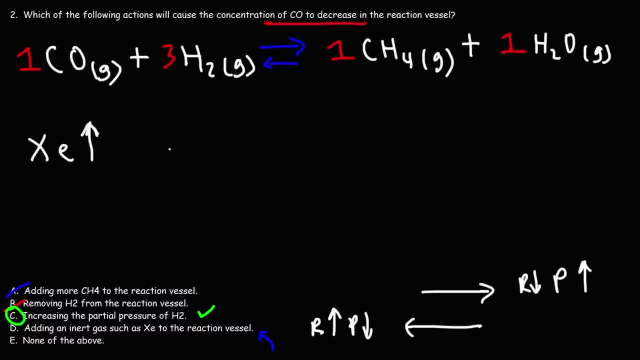 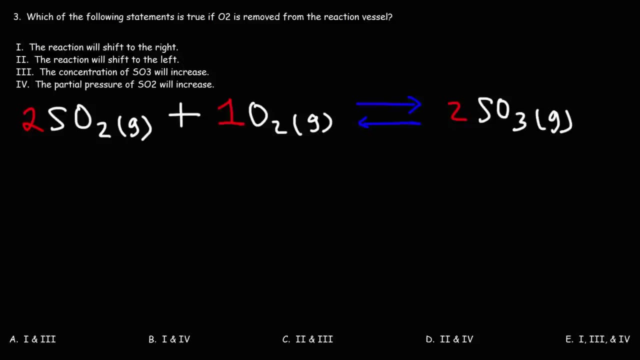 Therefore, the introduction of this inert gas will have no effect on the position of equilibrium. The reaction will not shift to the right, nor will it shift to the left. So C is the correct answer for this problem, Number 3.. Which of the following statements is true: 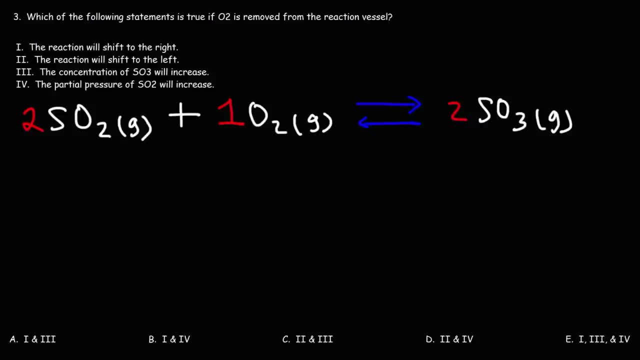 if O2 is removed from the reaction vessel. So if we decrease the concentration of O2, what will the system try to do to the concentration of O2? It's going to try to do the opposite. It's going to try to increase it. 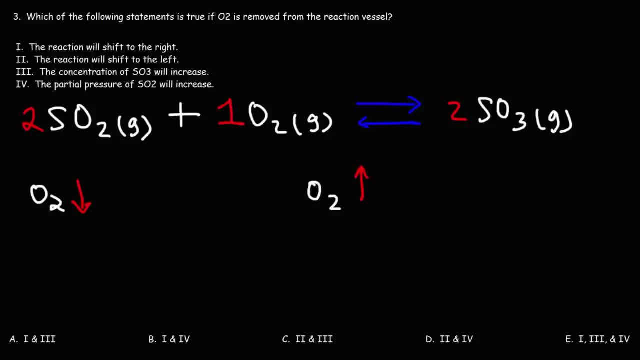 Now, in which direction will the reaction have to shift in order to increase O2?? Now, O2 is a reactant, So in order to increase the reactant, it has to shift towards the reactant. So the reaction has to shift towards the left, As it. 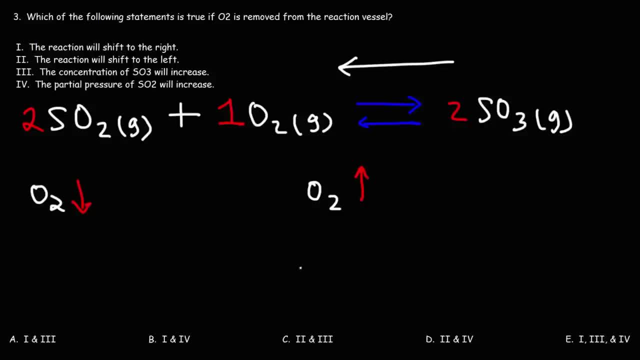 shifts towards the left. let me put this here: the concentration of all reactants will go up when it shifts to the left. So SO2 will increase in value and O2 will also increase in value, Which is what it's trying to do. 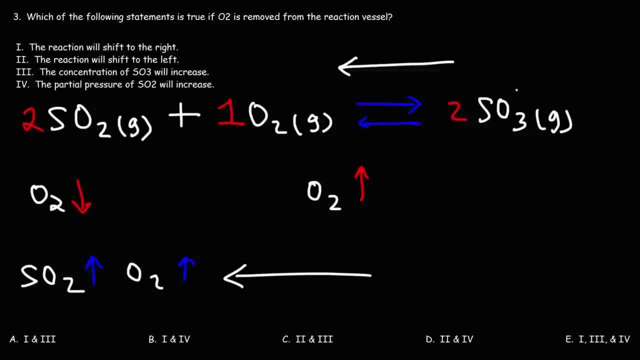 Now the reaction is shifting away from the products. So SO3 is a product Because the reaction is shifting away from it. the product will go down in value. So now we can find out which statement is true and which one is false. So number 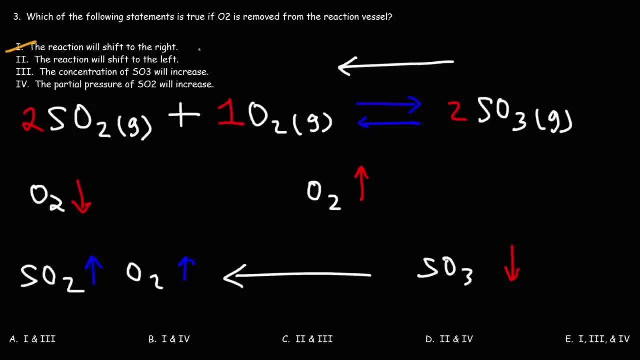 one. the reaction will shift to the right. That's false. We know it's going to shift to the left. So statement 2 is true: The concentration of SO3 will increase. That's false. SO3 is decreasing Because it's going to shift away towards it. 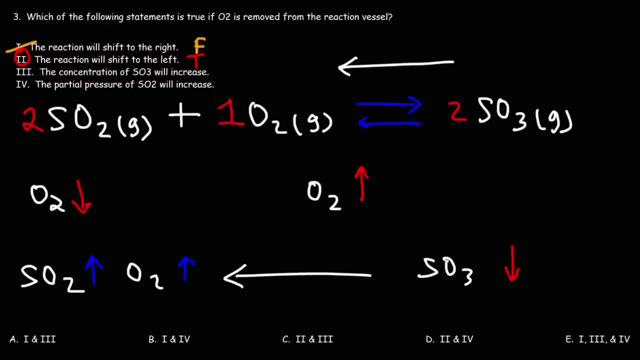 I mean it's shifting away from SO3.. So that's why it's decreasing. And number four, the partial pressure of SO2 will increase. That's a true statement- As the reaction shifts towards the left, towards the reactant. 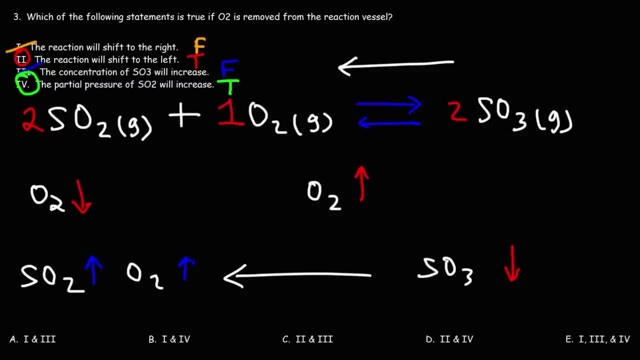 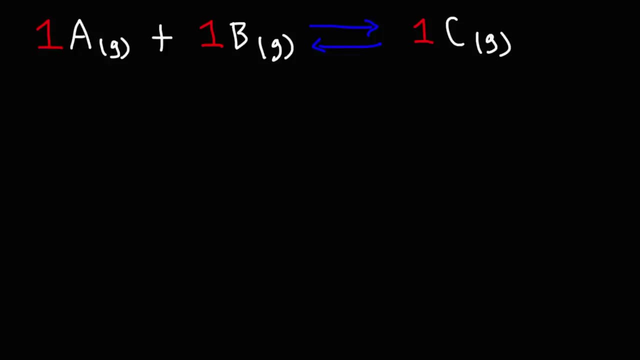 SO2, being a reactant, will increase in value, So both the concentration and the partial pressure of SO2 will increase. So only statements 2 and 4 are true. Therefore, answer choice D is the correct answer. Now let's move on to our next topic. 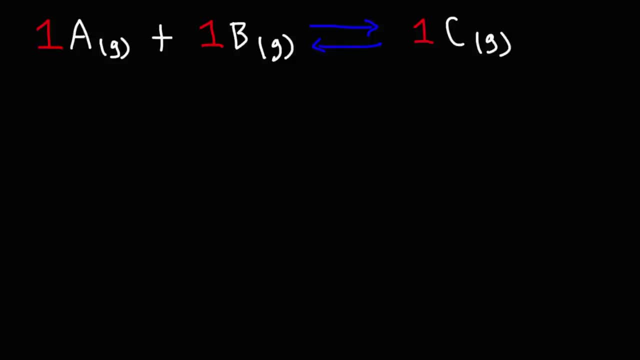 Let's say we have A reacting with B to produce C And everything is in the gaseous phase. What's going to happen if we increase the volume of the container? Will the reaction shift to the right or will it shift to the left? 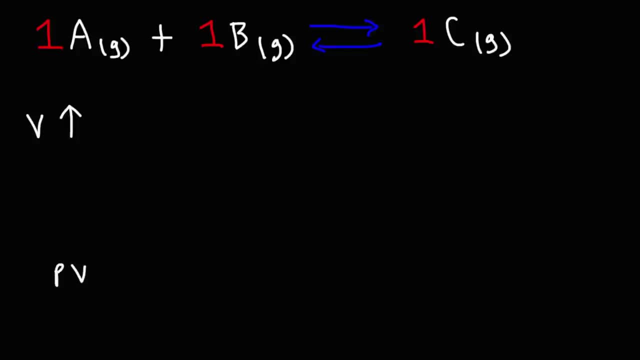 Now, if we think about the ideal gas law, PV is equal to nRT. If we divide both sides by V, we get that the pressure is equal to nRT over V. Notice that volume is in the denominator of that fraction. That means that volume and pressure. 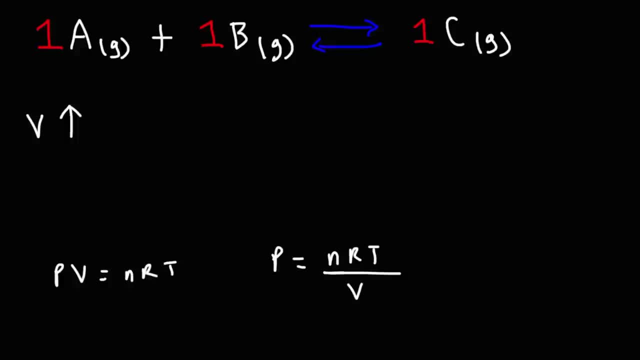 are inversely related. If you expand the container, if you increase its volume, the pressure is going to go down, And that is the total pressure of the system. Now what's going to happen if the total pressure decreases? Well, the system is going to try to increase. that total pressure. Whatever change you impose on the system, the system wants to undo that change. So if you decrease the total pressure of the system, it's going to try to increase it. Now, in which direction does the reaction have to shift in order to increase? 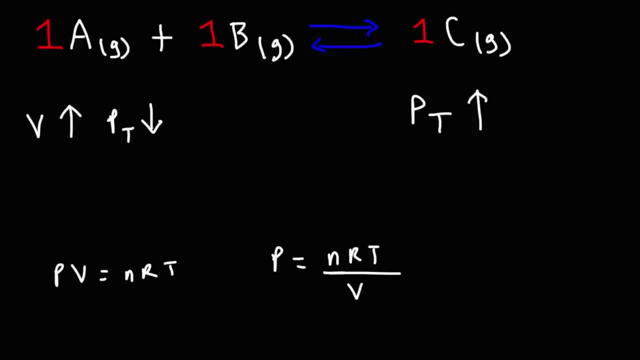 the total pressure, Should it shift to the left or to the right? Now notice that we have one gas molecule on the right side, but we have two gas molecules on the left. In order to increase the total pressure, it needs to shift to the side. 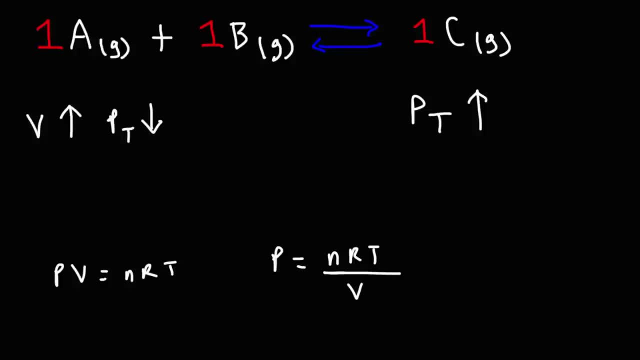 with more moles of gas molecules. So we have two moles of gas molecules on the right per one mole on the left. So it's going to shift to the left side because there's more moles of gas And by shifting to the left, 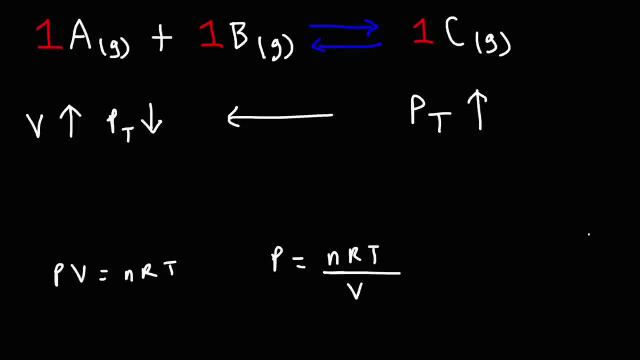 it's going to increase the total pressure. Earlier we said that as we increase V, the pressure decreases, since V is on the bottom, But N is an enumerate of that fraction. As we increase N, the pressure increases. So, in order to increase the total pressure, 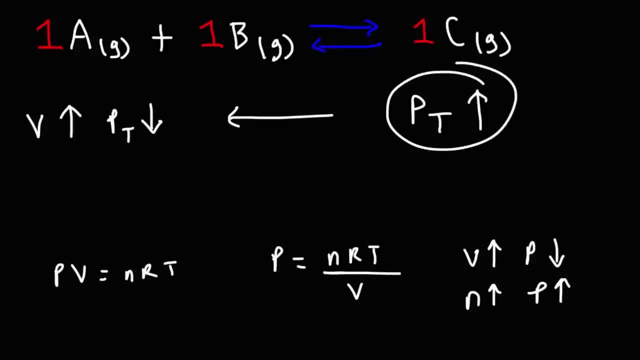 we need to increase the total moles. So when the system tries to increase the total pressure, it's going to go to the side with more moles of gas. There's a direct relationship between N and P. Now let's consider the reverse situation. 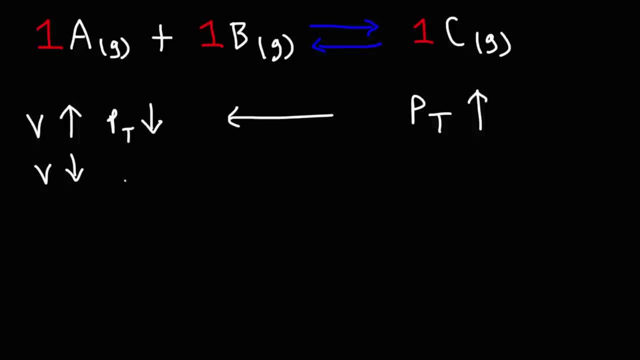 If we were to decrease the volume of the container, the total pressure will increase. Now the system will try to decrease the total pressure. So in order to decrease the total pressure, it needs to decrease the number of moles. There's a direct relationship between: 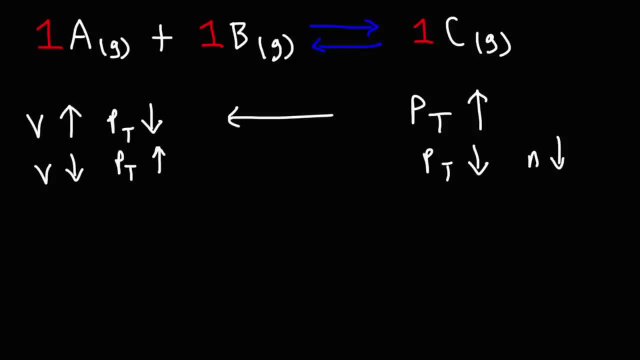 N and P And to decrease the number of moles, it has to shift to the side with less moles of gas. That is towards the right, Because there's less moles of gas there. Now let's understand more about this. 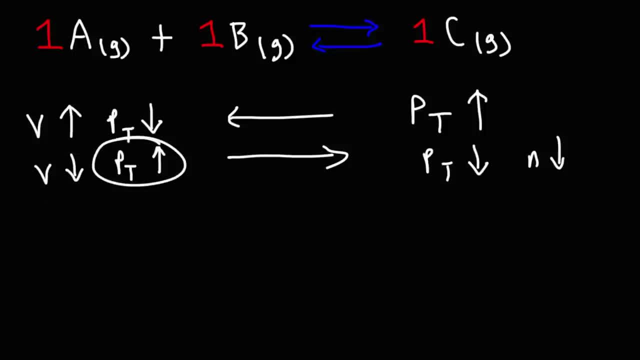 Because we described this in terms of the total pressure inside the container, But let's talk about it in terms of the partial pressure. So we're focused on the second situation. As we decrease the volume, the total pressure increases. That means the partial pressure of. 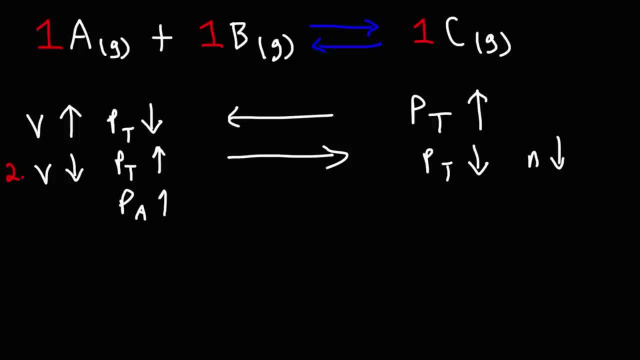 every gas increases, The partial pressure of A goes up, the partial pressure of B goes up and the partial pressure of C goes up. Now what happens if we increase the partial pressure of A? If you increase A, the system is going to try to decrease it. 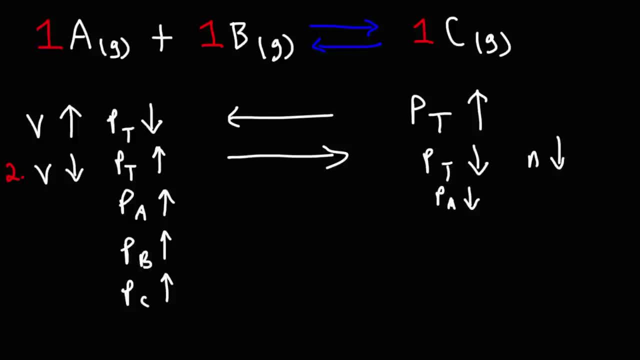 It's going to try to bring it down, And the only way that's going to happen is if the system moves away from A, So it's going to shift towards the right. Same thing for B. If we increase the partial pressure of B, the system 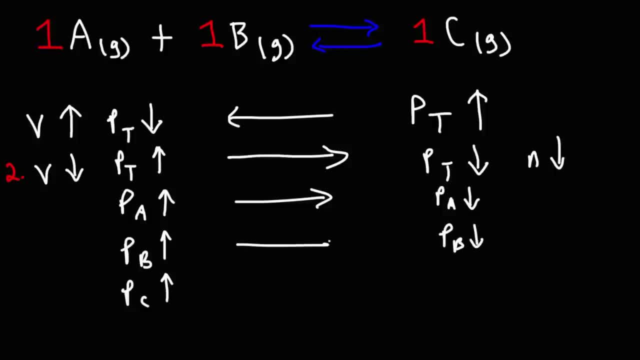 is going to try to decrease it, So it has to shift away from B to decrease the partial pressure of B As we increase the partial pressure of C. the system is going to try to do the reverse. It wants to decrease it, So it has to. 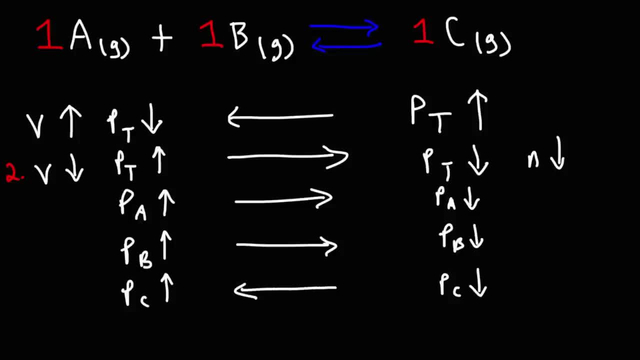 shift away from C, That is, towards the left. So notice that we have two arrows going towards the right, But only one arrow going towards the left. The net effect is that these two is going to win over this one. So two against one. the net result is that the 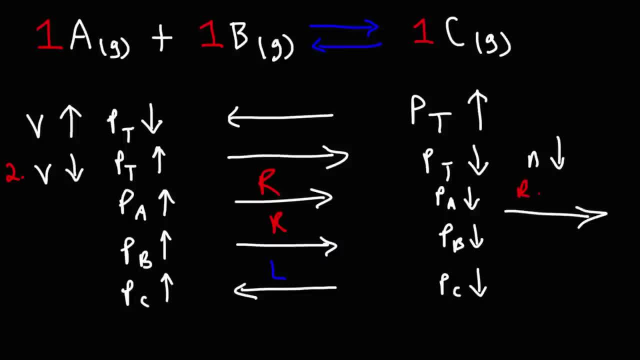 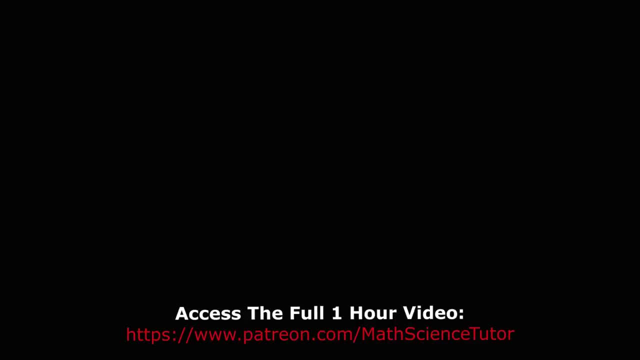 reaction is going to shift towards the right if we decrease the volume. Thank you for watching.